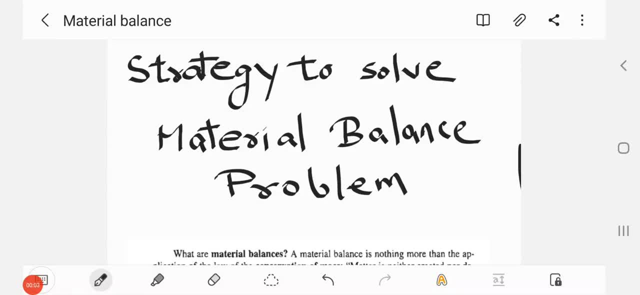 hello everyone, welcome to the channel. chemical engineer, I am Sahil Yadav and in this video we are going to continue our process- calculation syllabus- in which, in this video, we will be going to discuss about strategy to solve material balance problem. so now we are into material. 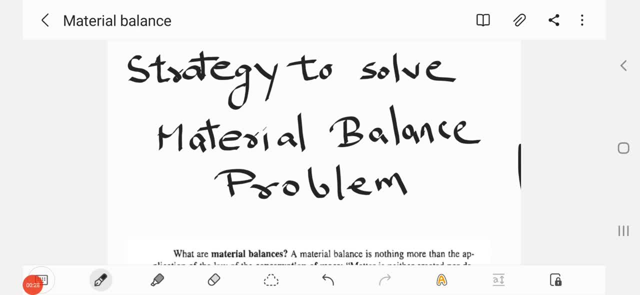 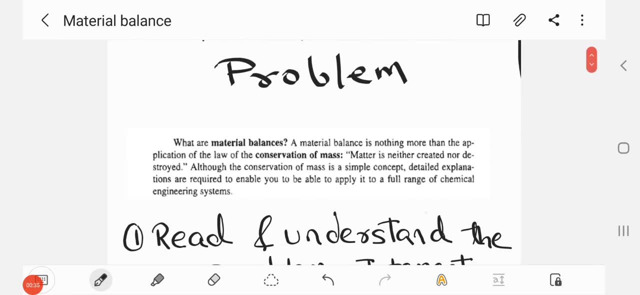 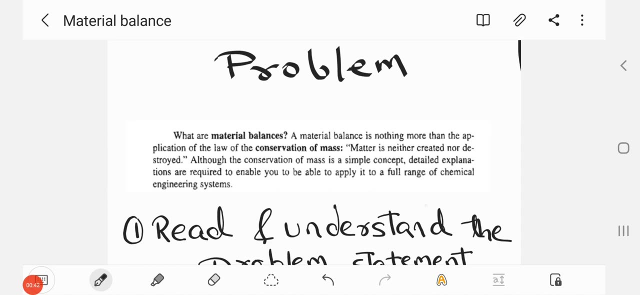 balance. so before going into how to solve any problem on material balance, you should know what is material balance. so a material balance X is nothing more than the application of law of conservation of mass. ok, so what does it mean? that anything can be balanced? make sure you understand Amsterdam and what is is just all broken down. 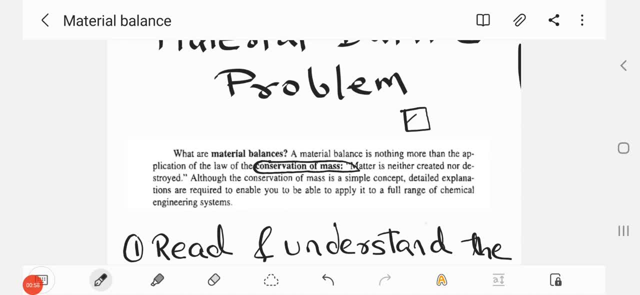 neither be created nor be destroyed. so that is simple enough. so anything which goes into the reactor will always comes out. so that is the basic principle of material balance. so if you are given any problem on material balance, you should follow steps to solve it. so the first step is read and understand the problem. 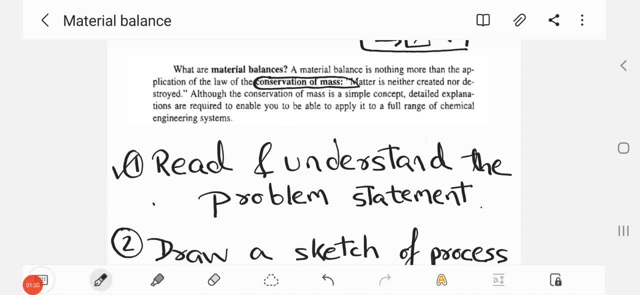 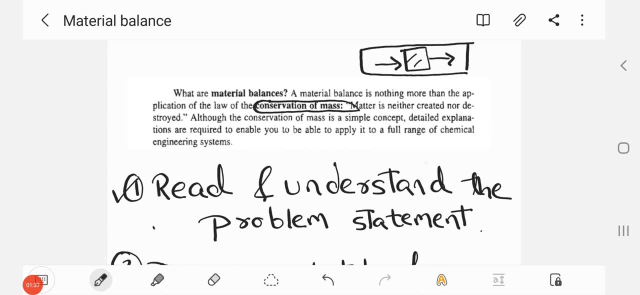 statement. okay, so I forgot to tell you that in this video, what we are going to do is we will see strategy to solve material balance problem, along with one example. okay, so please share this video you and please subscribe to the channel. alright, so the first step, you should. 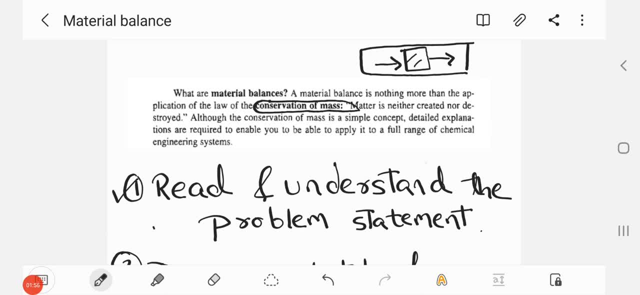 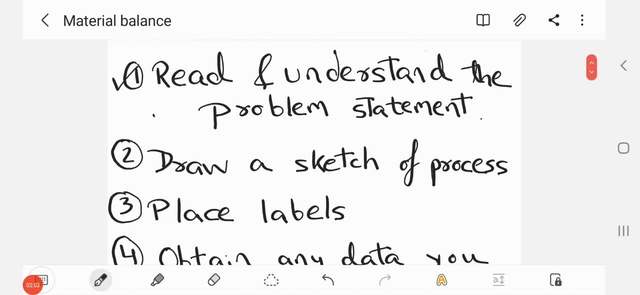 follow is understand the problem statement clearly. okay. second step you should follow is drawing the sketch of the process. sketch means you don't need to be an artist for that, but you should be able to draw such small block diagram. you should be able to draw such small block diagram. 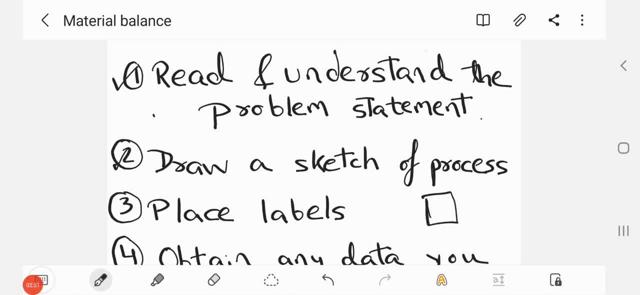 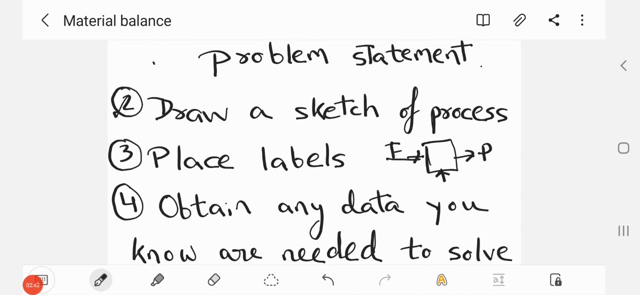 diagram, diagram. okay, so you should be able to draw small block diagram of inlet, outlet, another stream or like that. okay, so that is what required. so you should draw the sketch of the process. second point, third point: you should place the labels like: suppose this is fade, this is product, so you should name it as F, P and you know. 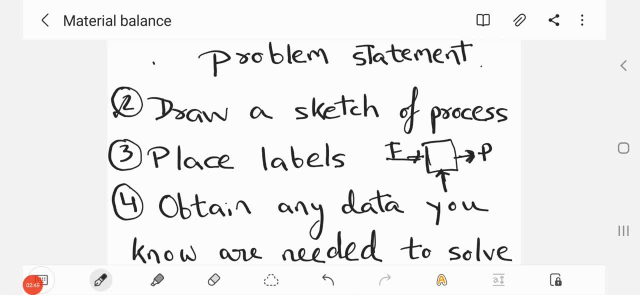 how to write or how to write a product, and you know how to write or how to give label. so on the top of arrow you should write P. on the top of inlet arrow you should write F. suppose this is some other stream. let us name W and suppose. 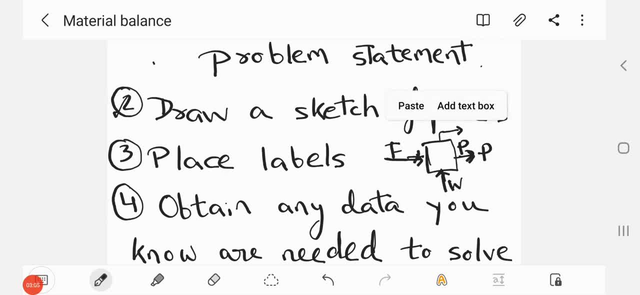 this is also a stream, latest name as okay, so you should name the stream based on the arrows and other things like composition. you should write a fiber layer so in order to understand how to below arrow like this is 0.5, this is also 0.5. suppose this is x1, this is x2. so on that we will. 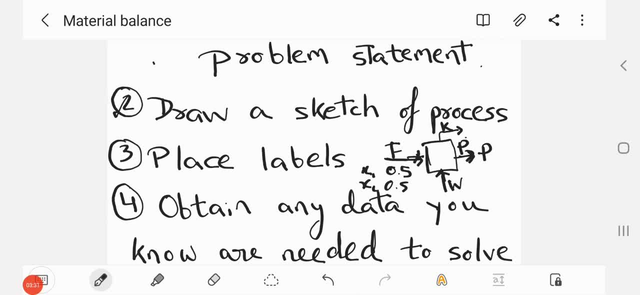 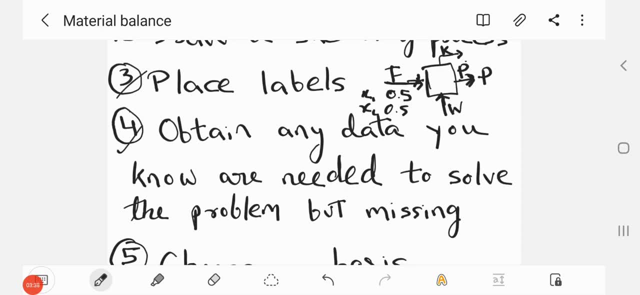 go through when we are solving a problem. so third thing is place a label. fourth thing you should do is obtain any data if you are needed and which is not given in your problem, so you can refer to the standard tables or online if possible. so if such data which are required, like suppose, 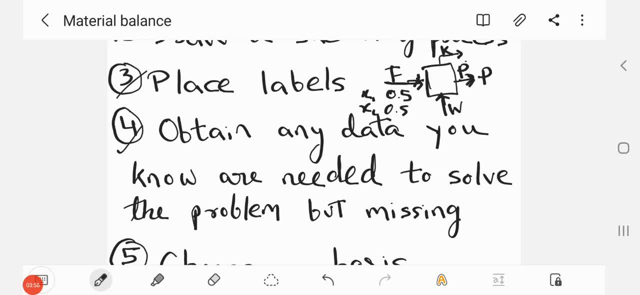 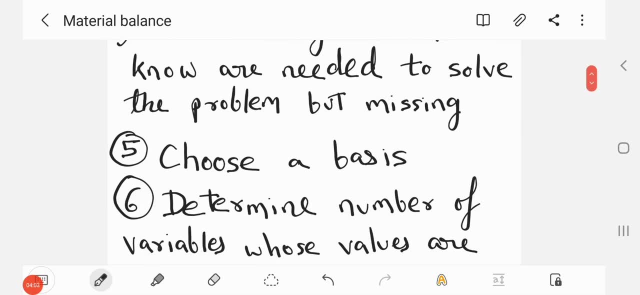 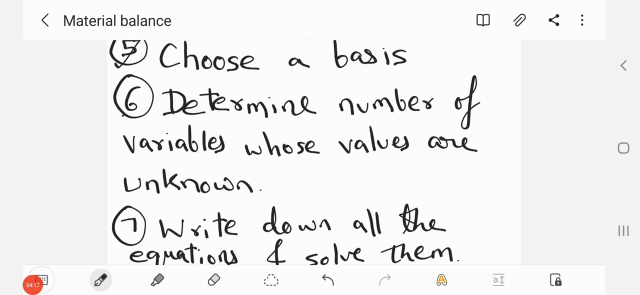 partial pressure is not given at certain temperature, then you can refer tables or standard data. fifth is choosing a basis. so this important part is already covered. how to choose a basis in the previous videos. refer it, then determine the number of variables whose values are unknown means you have to find out. 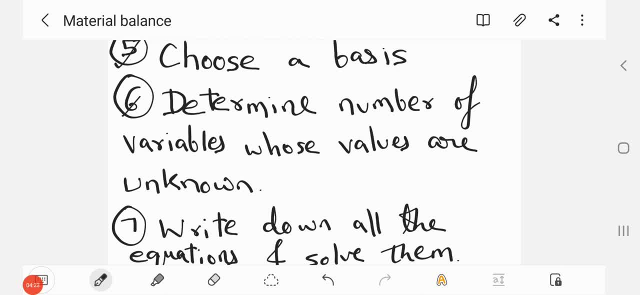 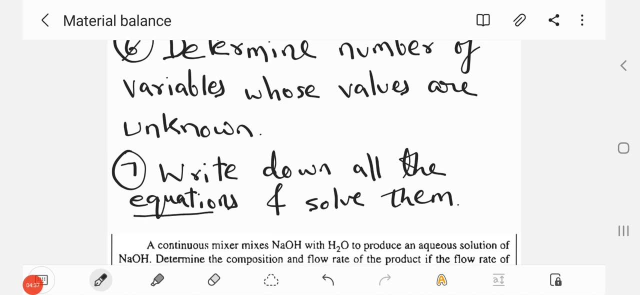 or list out the variables or quantities which are needed to be find out in your question. okay, so you should know that which things are to be find out and how to find out. so how to find out, you have to write down the equation and solve them. okay, so basically four steps to be followed. 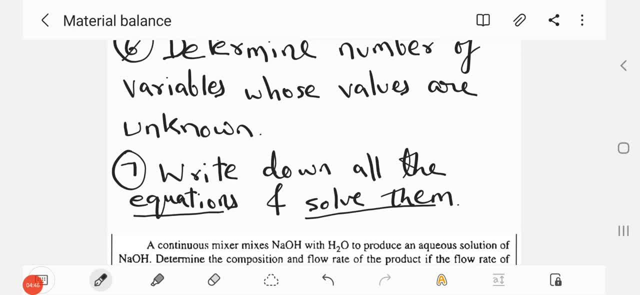 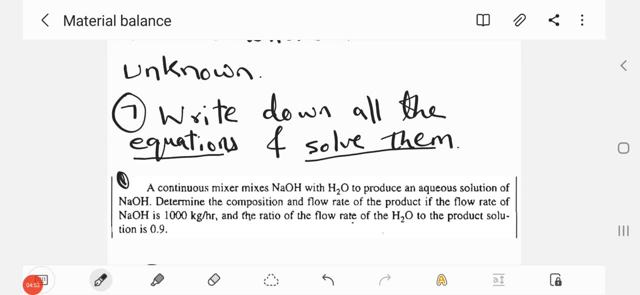 now let us see an example of it. all right, so this is a quotient that we are going to solve. so what quotient speaks is: a continuous mixture mixes NaOH with H2O to produce an aqueous solution of NaOH. I hope this line is clear. 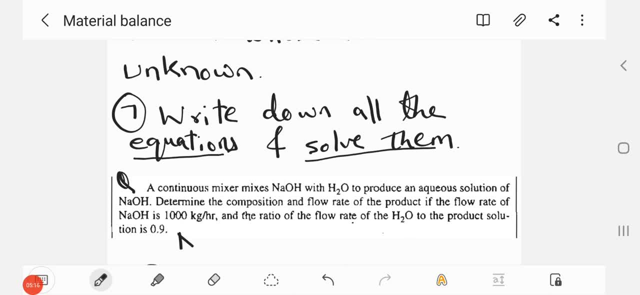 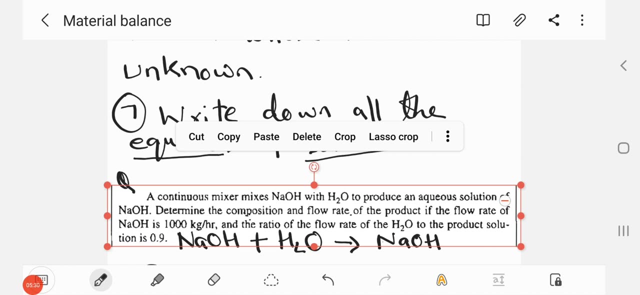 E4. So what we are doing- mixing of NaOH with H2O- and what we are getting- aqueous solution that is NaOH only, but in aqueous phase. okay, or you can write it as NaOH dot H2O. So that is So. that is what we are getting as our final product. 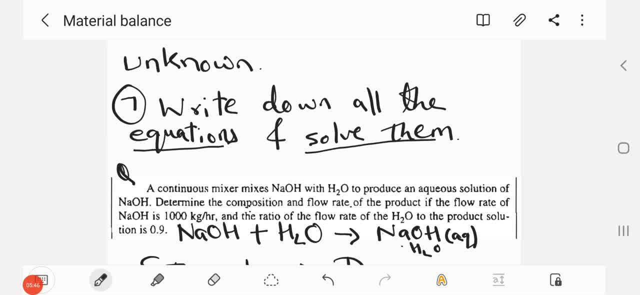 so first line is clear: we are doing this in mixture mixer. now what we are needed to find out is determine the composition and flow rate of the product. third name is product. so our product is this aqueous solution, this is our feed, this is our binary, or we can say utility that we will. 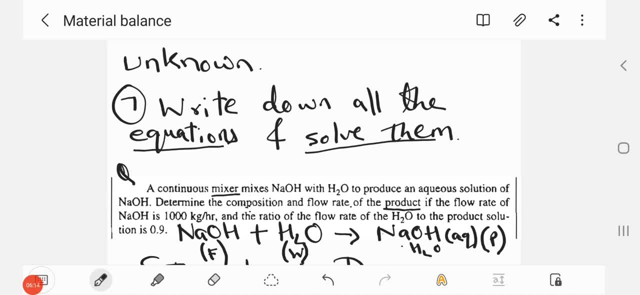 be required. let us name as W for water, and final product is P, that is, product. if the flow rate of NaOH is thousand kg per hour and ratio of flow rate of h2o to the product, solution is 0.9. so these two data's are given to us. now let us go step wise. so first step is: 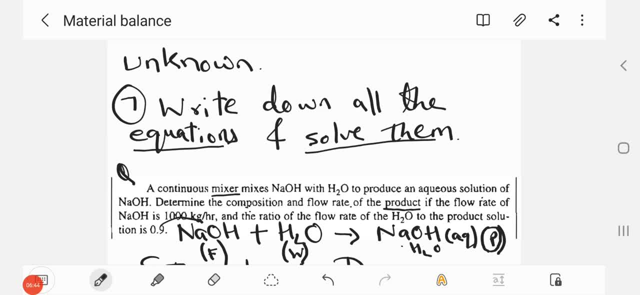 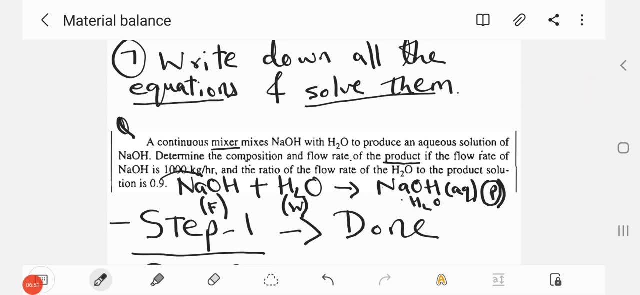 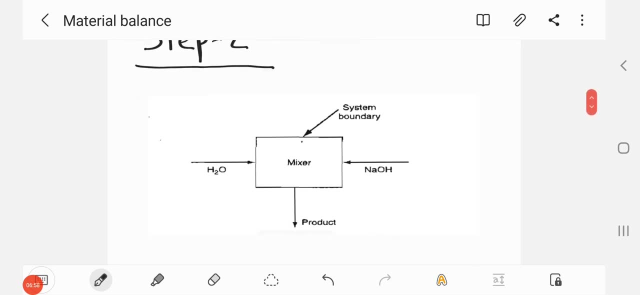 we are going to determine the composition and flow rate of the product. third line is clear, we are clear. you have read and understood the problem statement clearly. okay, so Step one is done. so step 2 is sketching of the process. so let us do the sketching. 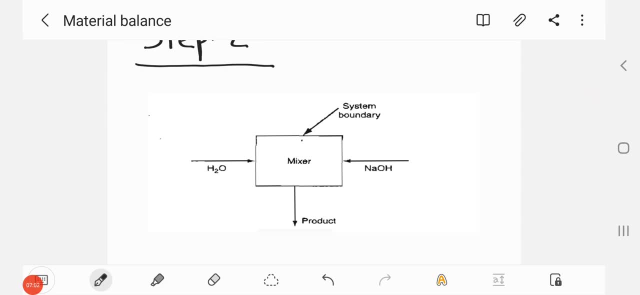 so this is how we will sketch the product. so we have h2 of going in let to the mixer, NaOH going to the mixer and product coming out through the mixer. you can draw it anyway, like you can add here NaOH or anywhere. you can draw NaOH or like. 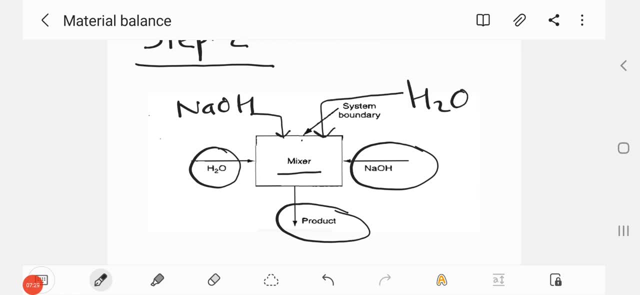 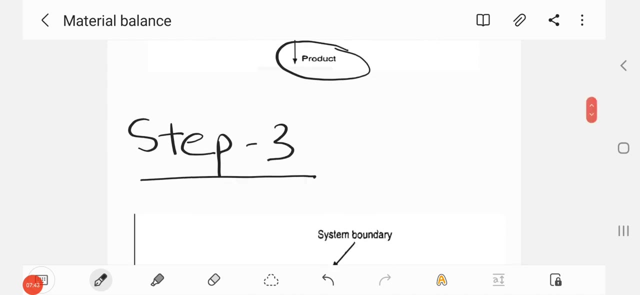 you can draw here H2O, anywhere you can draw, but you should understand it clearly. so this is what our basic block diagram, or the sketch of the process, looks like. step 3 is to place a labels. so what things is given. so we are given the feed flow rate, that is 1000 kg per hour. okay, so we can write it here: feed. 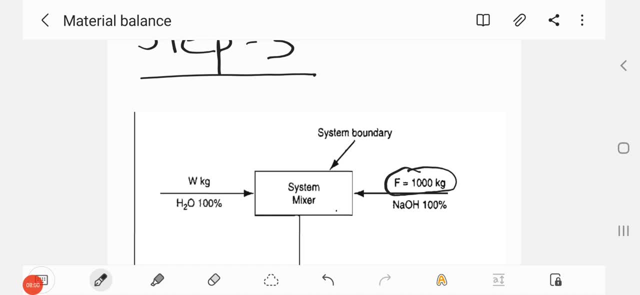 as F, equal to 1000 kg per hour, and we are given percentage. so here in this stream we are adding only NaOH, so we are adding only NaOH. so we are adding only NaOH, so this stream contains only NaOH. so we are writing NaOH as 100% NaOH is. 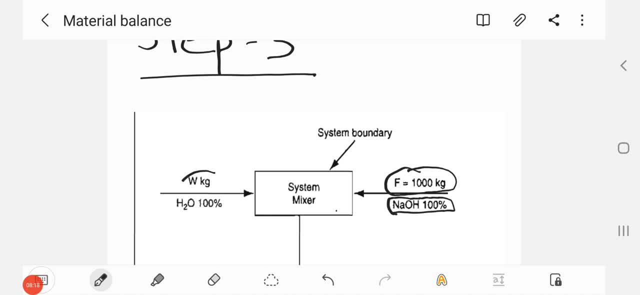 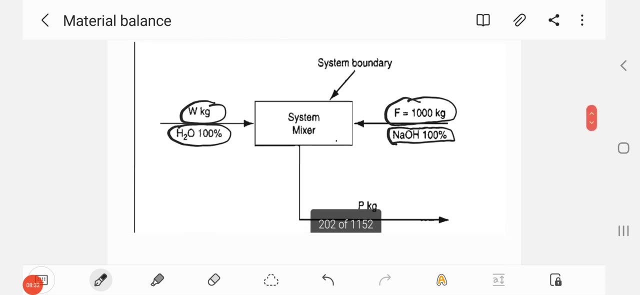 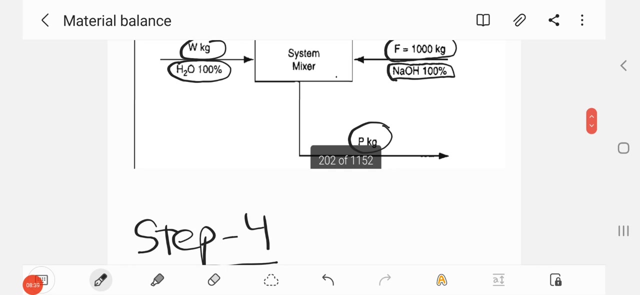 going through this F. second is W, whose value is not known to us, and H2O, 100%. okay, we are feeding H2O purely through this stream and this is for product, whose values will be found out. okay, we are leading this flow rate and we Marriage devong form and this will 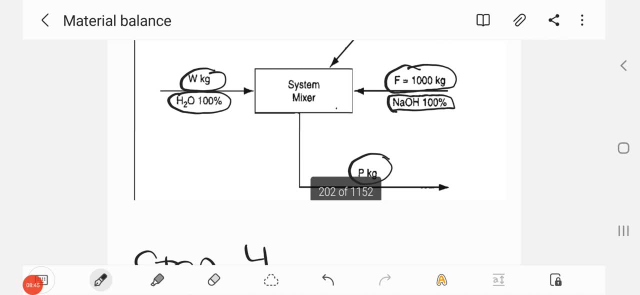 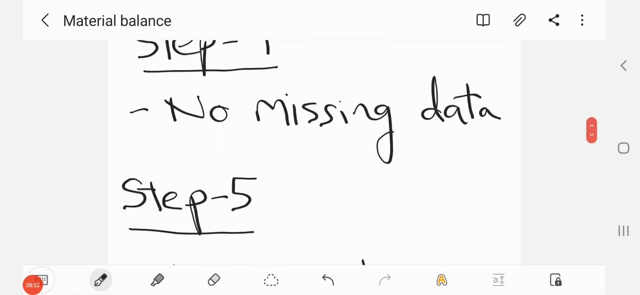 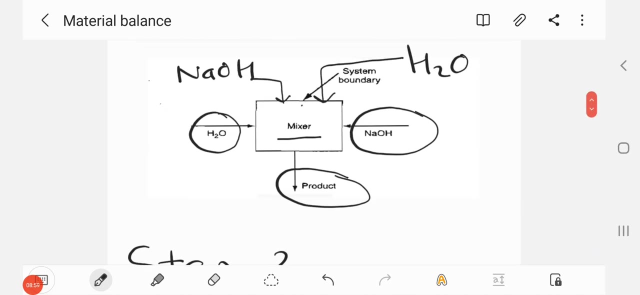 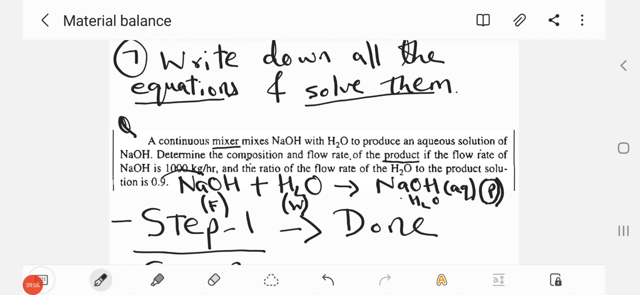 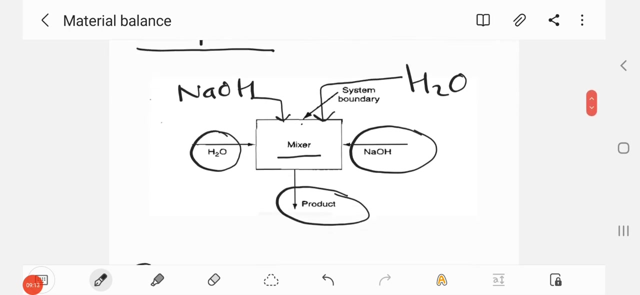 interact with each other. so step 4 is moving from Tjets below ans смотреть naoh. moving to next step of the psychologist. so save. moving to next step of the psychologist, so refer to the basis video, and here we are taking one hour operation as our basis. 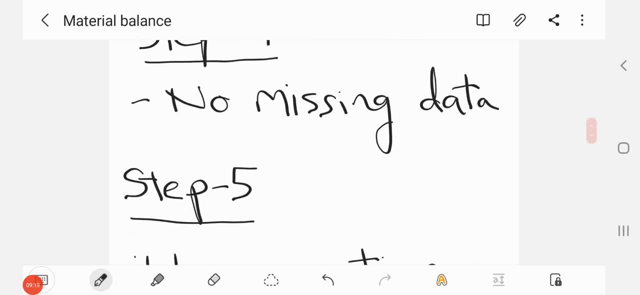 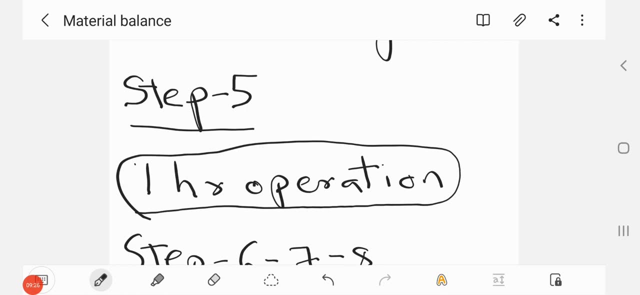 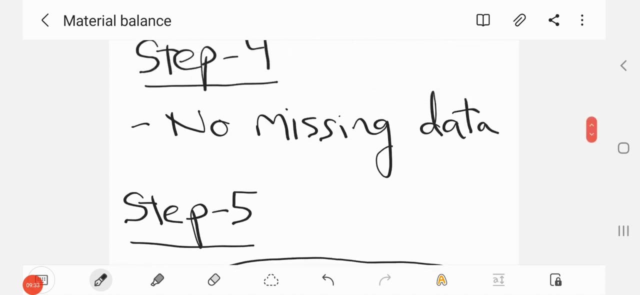 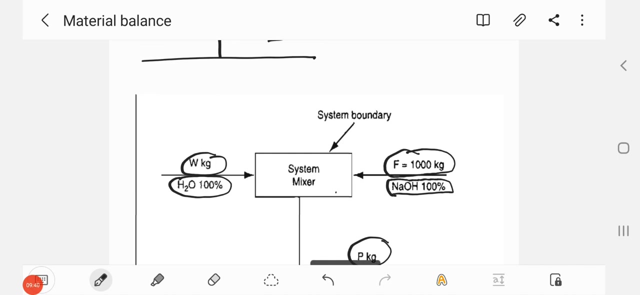 why we are taking you should know by now. so one hour operation is our basis. now step six, seven, eight, we will do solution by writing down the equations. so from this figure you can clearly say that whatever going in should come out. so what things are going in is f and w should always come out. so this should be equal to p. 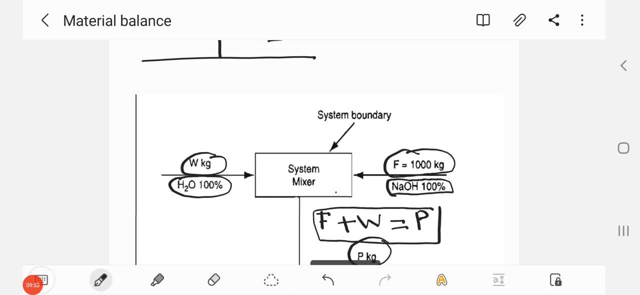 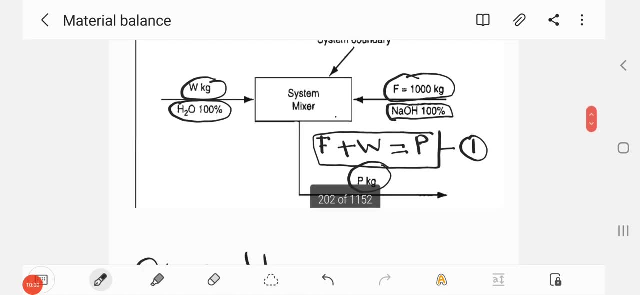 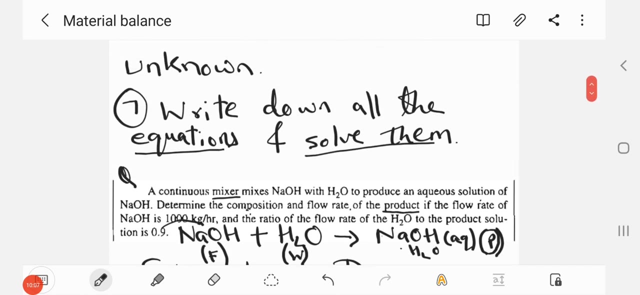 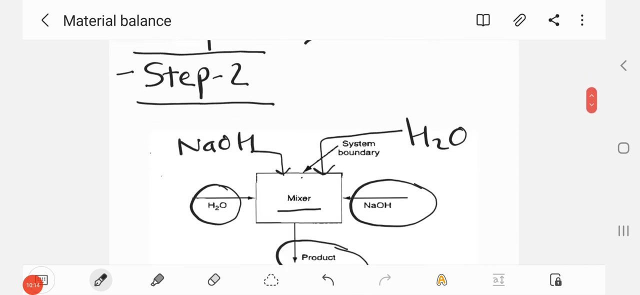 so this is the first equation that we will be getting. moreover, in quotient, you are given. the class is okay, so the what was given, W by P, is given, I think, the flow rate okay. so the ratio of flow rate of H2O to the product solution is 0.9. so W by P is given to you. so what is given as W. 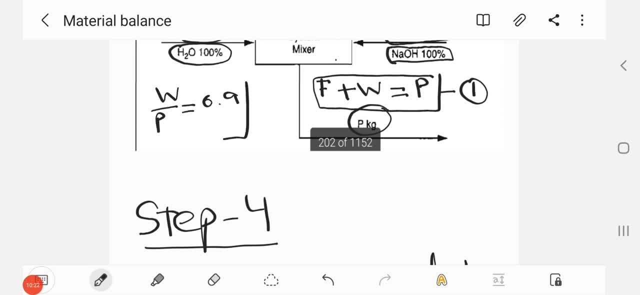 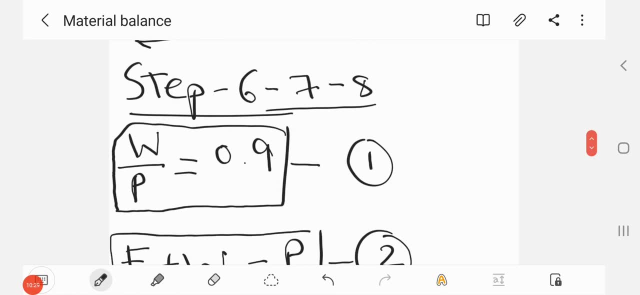 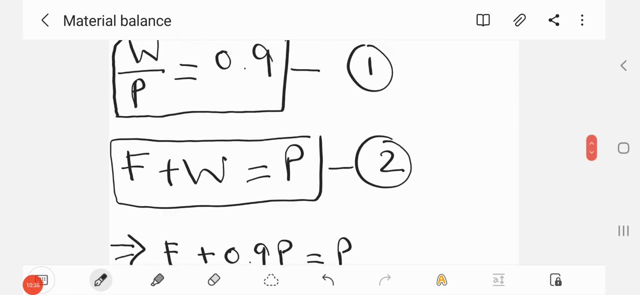 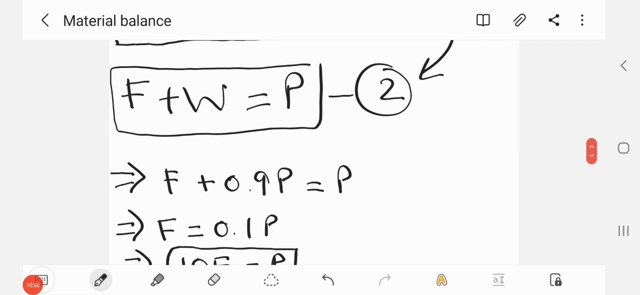 by P is equal to 0.9. so these two equations can be formed easily. so that is what we have formed: W by P is 0.9 and F plus W equal to P. so, solving this equation, we can put W equal to 0.9 P in equation number 2. that is what we have kept: F plus 0.9 P equal to P. so if 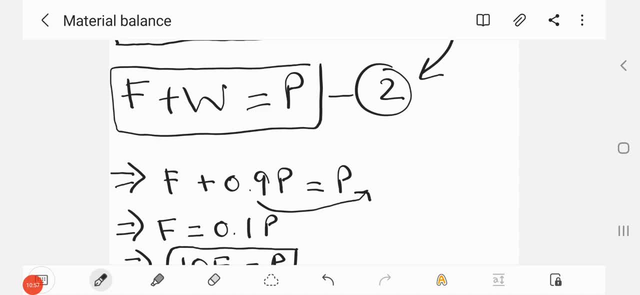 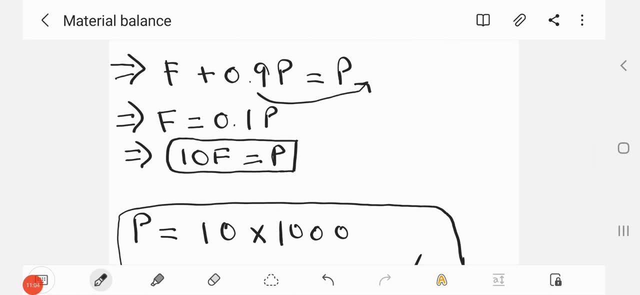 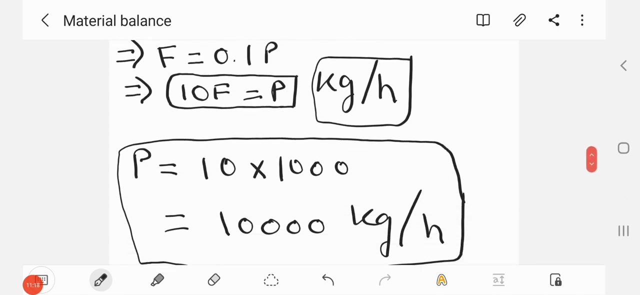 this goes to the right hand side- what we will get: F equal to 0.1 P Or F multiplied by 10, 10 F equal to P. so all these things we are doing for flow rate, kg per hour- remember units are important, so F is already given to us, that is, 1000 kgs per. 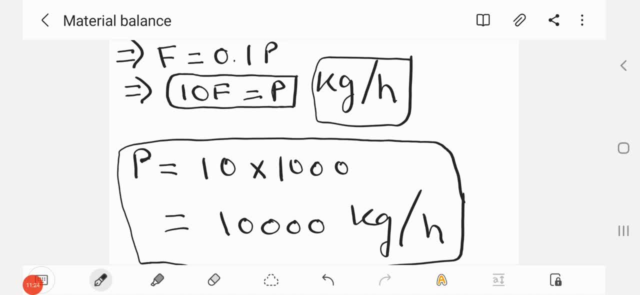 hour. so P can be found out directly as 10 multiplied by F. so F is 1000, so 10 multiplied by 10.. F multiplied by 1000 will yield to 10000 kgs. as we have taken basis as 1 hour, so we can. 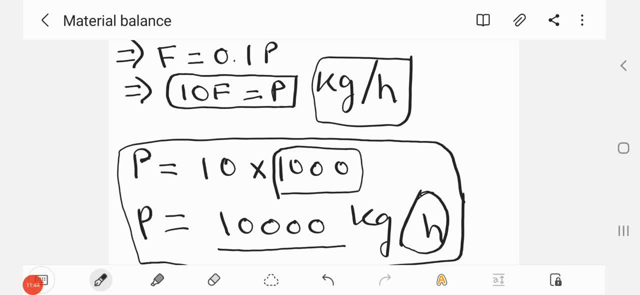 neglect it. so our product will have 10000 kg of product or flow rate if we are asking. so 10000 kg per hour is our required answer to the first question. 2. The composition of material balance. The second question is to determine the composition. 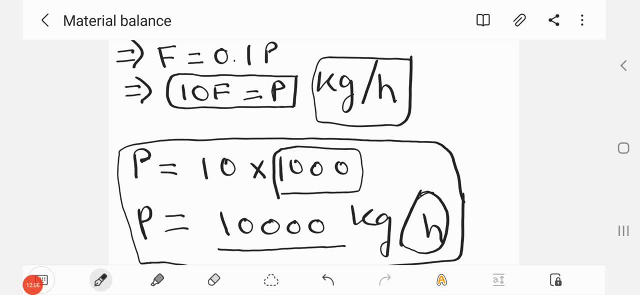 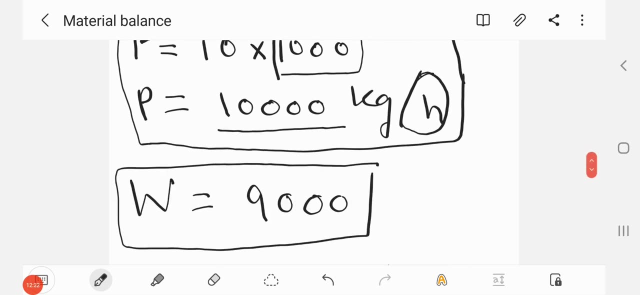 So, in order to determine the composition, What we have to do, we have to do material balance. So this is a question in which we are doing material balance without chemical reaction, because there is no reaction taking place, just mixing. Okay, Ok, So if we have found out, PW can be found out as 0.9 into. 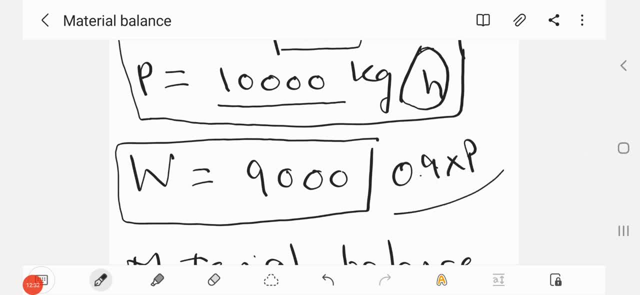 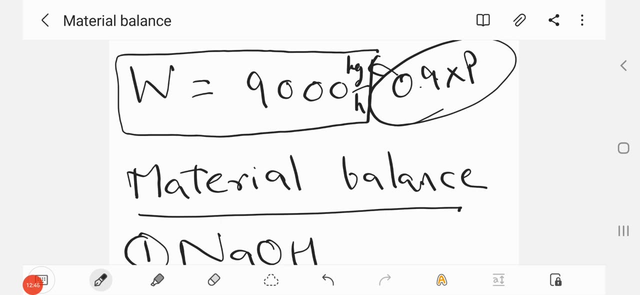 PW: 0.9 x, 0.9 x, 0.9.. 0.9 into P, so that is how we will find WS. 9000. unit should always be returned kg per hour. all right now, in order to find out the composition, what we will do. 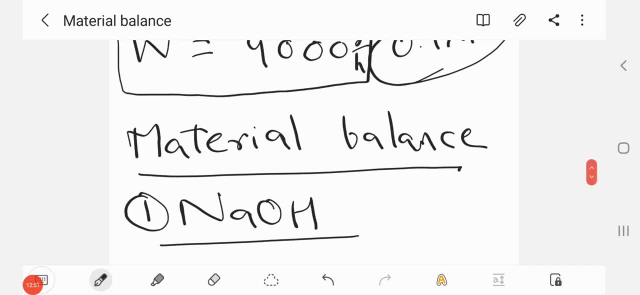 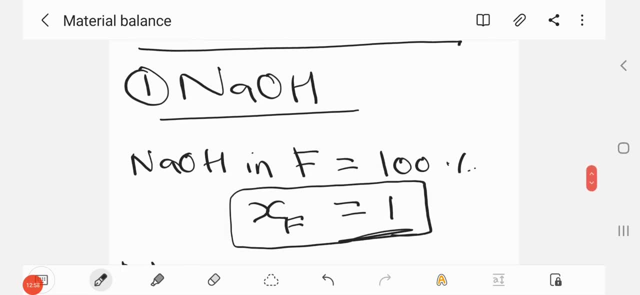 material balance. so first of all we will do material balance for sodium hydroxide, NaOH. okay, so NaOH in feed is hundred percent. so we can write the composition of feed F. XF is one, purely NaOH. okay, so that is one. you should know that XF ranges from zero to one. okay, so purely NaOH is going in F. so 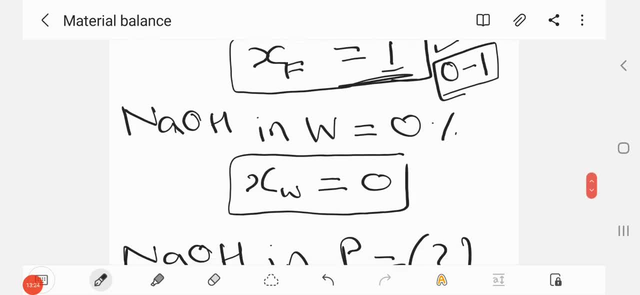 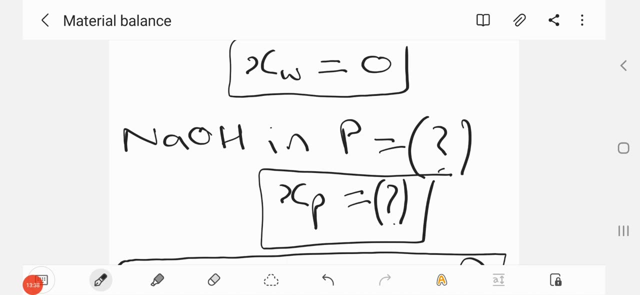 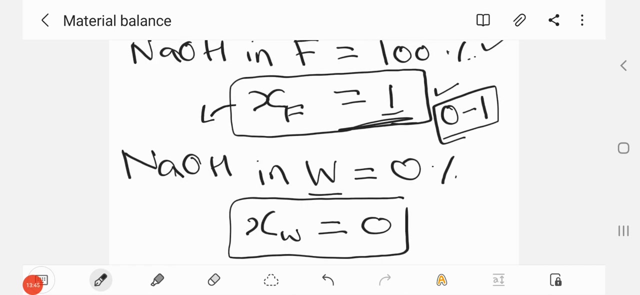 we can write XF equal to one, now NaOH in W string, so it is zero percent. so we can write: XW is zero. now we have to find NaOH concentration in product XP. that we have to find. okay. so what we will do is this composition, that is, composition multiplied by flow rate. 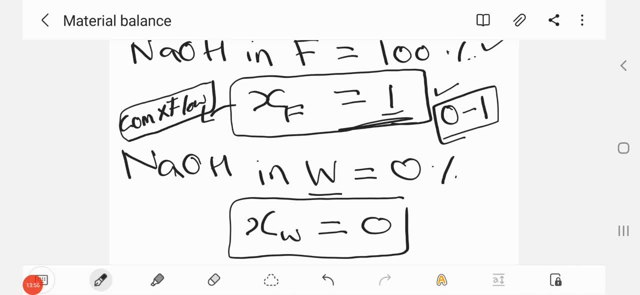 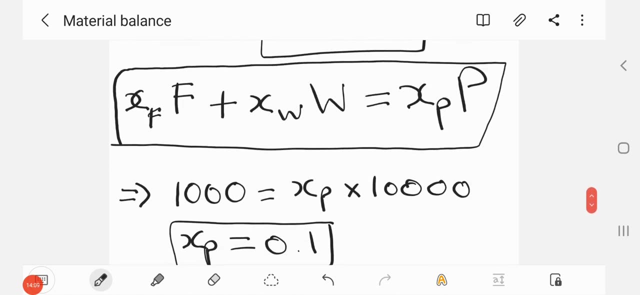 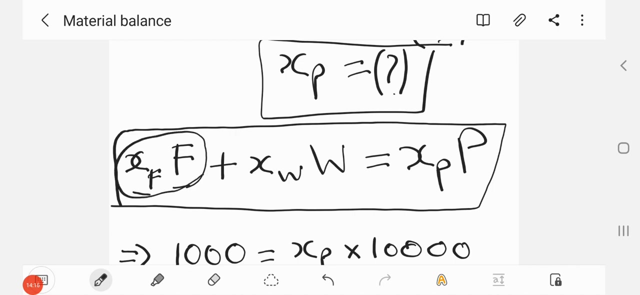 okay, okay. so this should be equal because we are doing material balance. everything going into the system should come out. so for a, now it's going into, the system should always come out. alright, so XF, x, f is for n o, H in the feed, F stream x.